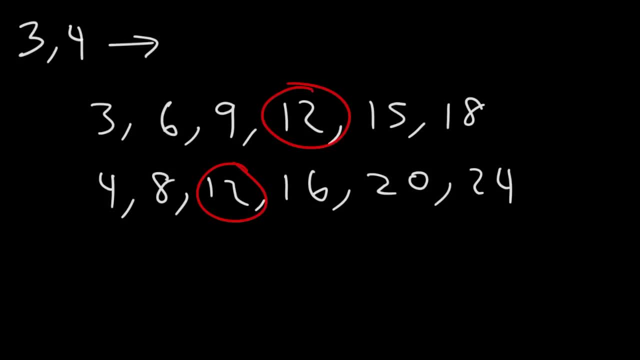 twelve is the least common multiple of three and four. Let's try an example with larger numbers. What is the LCM of 12 and 16?? Go ahead and try that. So common multiples of- I mean multiples of 12 rather- are 12,, 24,, 36,, 48,, 60, 72. 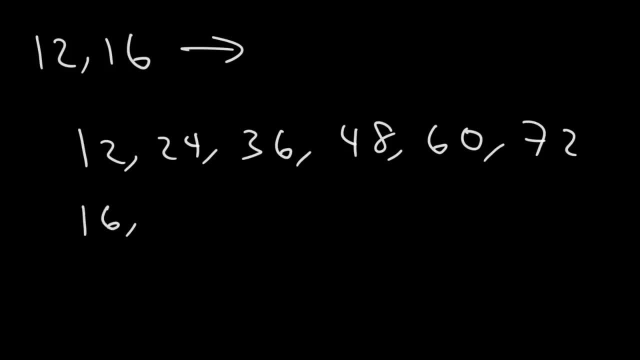 Multiples of 16 are 32,, 48,, 64 and 80. So the least common multiple of 12 and 16, we could see is 48.. Forty-eight is the lowest number that is divisible by 12 and by 16.. Forty-eight divided: 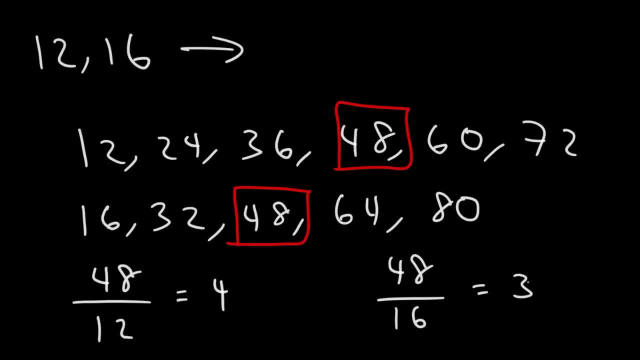 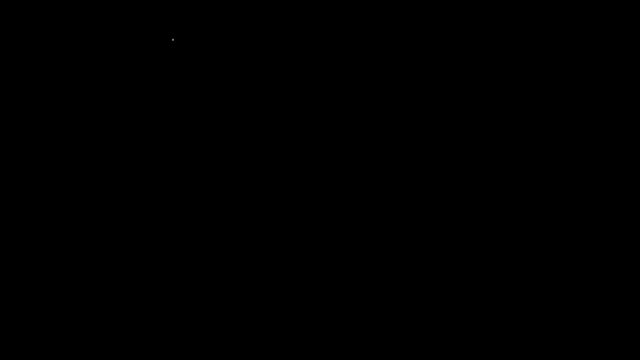 by 12 is 4.. And if you divide it by 16, you'll get 3.. So the LCM of two and three is six, So the LCM of, So the LCM is 48.. Now let's try an example where we have three numbers. 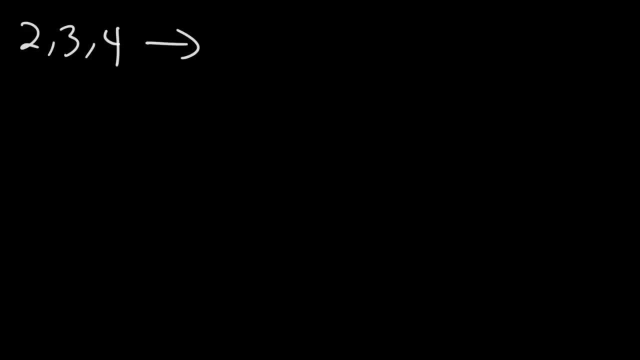 Let's say 2,, 3, and 4.. What is the LCM of those three numbers? Let's write out the multiples of 2.. So we have 4,, 6,, 8,, 10,, 12,, 14.. 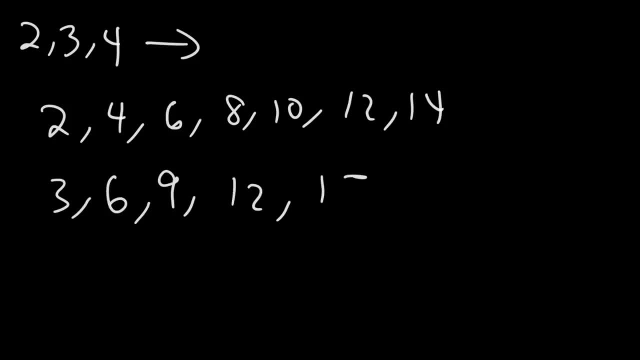 Numbers of 3 are 6,, 9,, 12,, 15,, 18.. And then, for 4, we have 8,, 12,, 16,, 20, and 24.. So, looking at these three lists, what is the LCM of 2,, 3, and 4?? 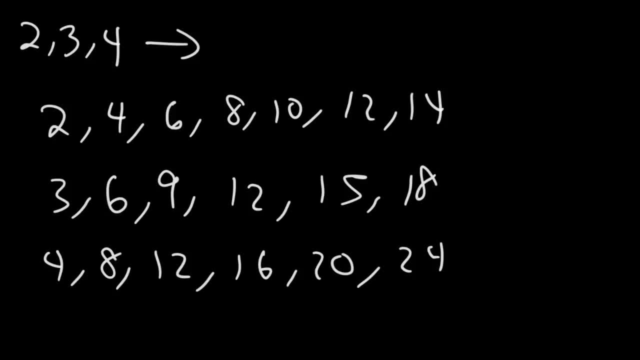 What is the least common multiple of these numbers. So we can see that 12 is the lowest number that is found in each list. So we can see that 12 is the lowest number that is found in each list. So the LCM of 2,, 3, and 4 is 12.. 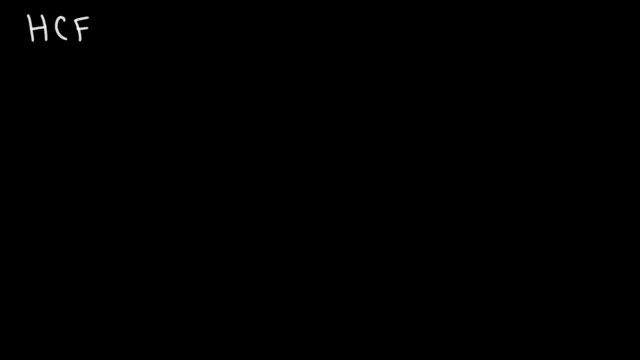 Now the next thing we're going to talk about is how to find the HCF. The HCF stands for the highest common factor. This is the same as the GCF, which is known as the greatest common factor. So let's start with a simple example. 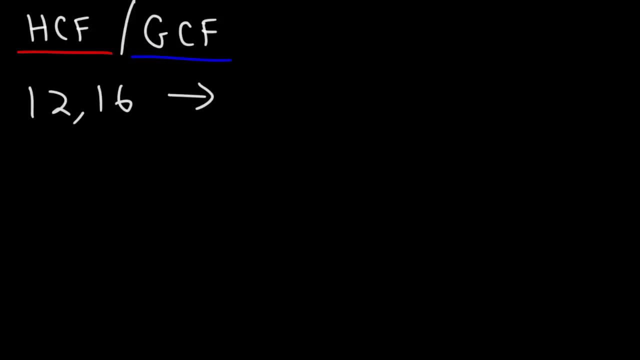 Let's use 12 and 16.. So what is the HCF of 12 and 16?? So let's write out the factors of 12.. Numbers that can go into 12 are 1,, 2,, 3,, 4,, 6, and 12.. 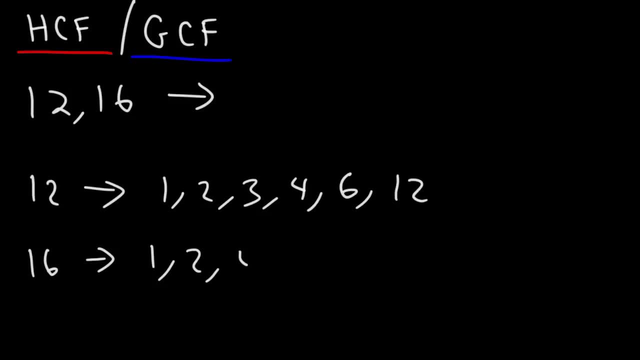 Now the factors of 16 are 1,, 2,, 4,, 8, and 16.. So 16 is divisible by all of those numbers. Now what is the highest number that is found in both lists? The highest factor found in each list is 16.. 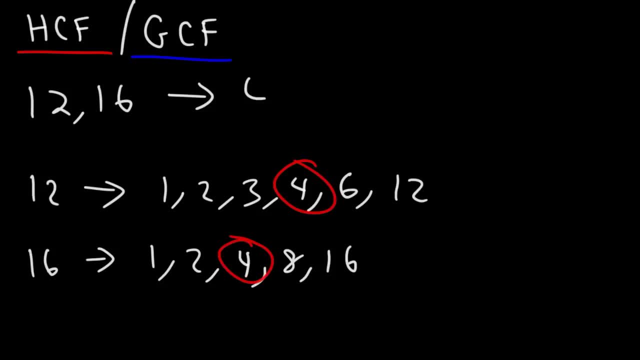 Which list is 4?. So the HCF of 12 and 16 is 4.. Now let's try another example. What is the HCF of these two numbers, 24 and 30?? Go ahead and work on that example. 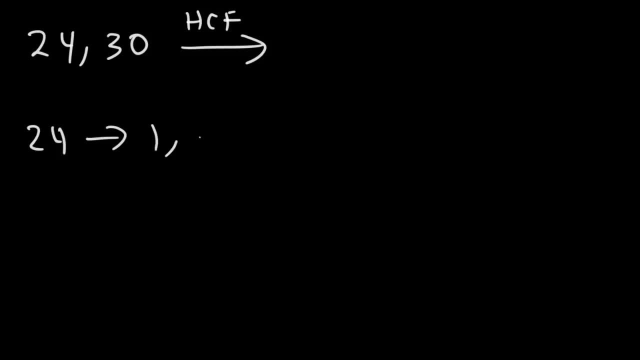 So let's write out the factors of 24.. So 1 can go into 24,, 2 can go into it, 3,, 4,, 6,, 8,, 9,, 10.. 8,, 12, and 24.. 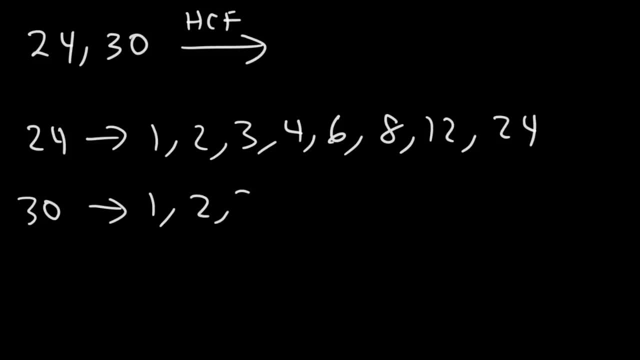 Factors of 30 are 1,, 2,, 3,. 4 doesn't go into 30, 5 does 6,, 7,, 8, and 9,. they can't go into 30. You can't divide 30 by 7,, 8, and 9 and get an integer. 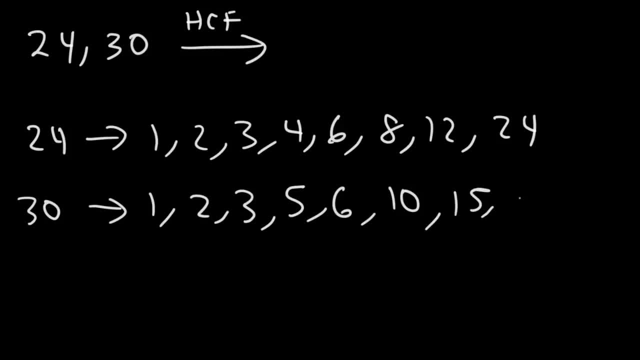 You could divide it by 10,, you'll get 3.. 15 is a factor of 30, and so is 30. So now the highest common factor in these two lists: It's 6.. That is the highest factor that can be found in both lists. 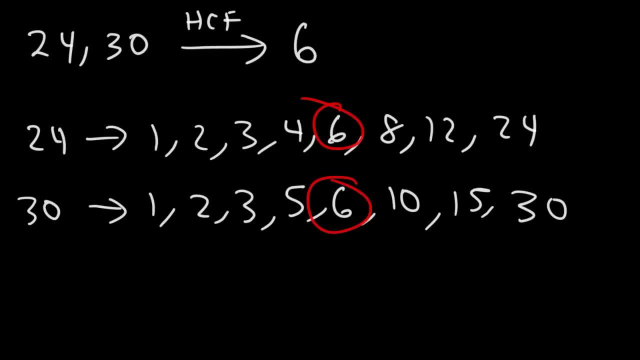 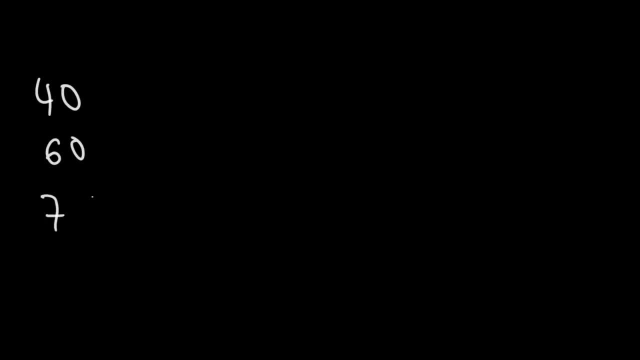 So that's the HCF for 24 and 30.. Now let's try three numbers: 40,, 60, and 75.. Go ahead and find the HCF of those three numbers. So let's begin with 40.. So we have 1,, 2,, 4 can go into 40. 5,, 6,, 7,, 8,, 9,, 10.. 5, 6,, 7,, 8,, 9,, 10.. 5,, 6,, 7,, 8,, 10.. 5,, 6,, 7,, 8,, 9,, 10.. 4,, 1,, 2,, 3,, 3,, 4,, 4,, 5,, 4,, 4,, 5,, 6, and 7. doesn't go into 40..